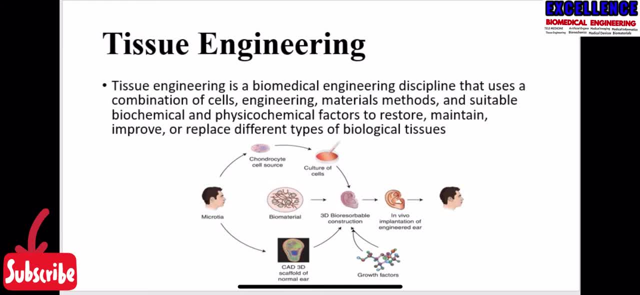 like to first give a brief definition of tissue engineering. Well, tissue engineering is a biomedical engineering discipline that uses a combination of cells, engineering material, methods and suitable biochemical and physical chemical factors to restore, maintain, improve or replace different type of biological tissues in the human body. So that is why 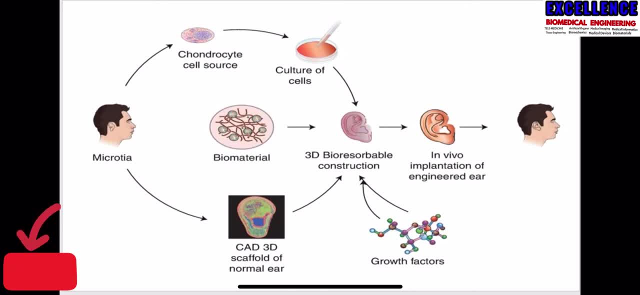 our primary example here is that of someone who lost his earlobe, maybe due to a war or due to an accident, or maybe some certain disease, If someone happened to have got his earlobe cut out or damaged. so with the help of tissue engineering- as you can see from this diagram here- is that chondroblast source will be removed from the earlobe. So that is why tissue engineering is a biomedical engineering discipline that uses a combination of cells, engineering material methods and suitable biochemical factors to restore, maintain, improve or replace different type of biological tissues in the human body. So that is why tissue engineering is a biomedical engineering discipline that uses a combination of cells, engineering material methods and suitable biochemical factors to restore, maintain or replace different type of biological tissues in the human body. So that is why tissue engineering is a biomedical engineering discipline that uses a combination of cells, engineering material methods and suitable biochemical factors to restore, maintain or replace different type of biological tissues in the human body. So that is. 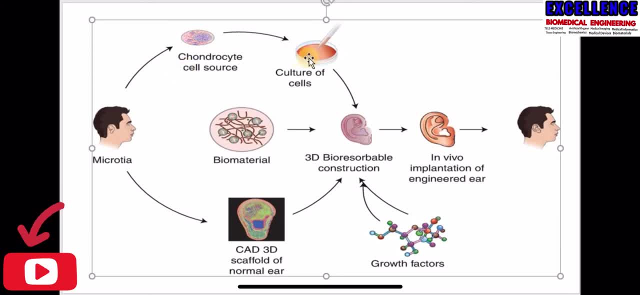 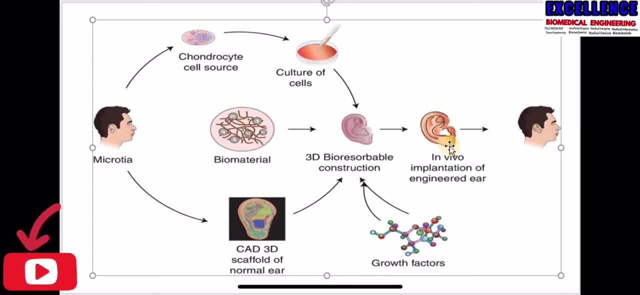 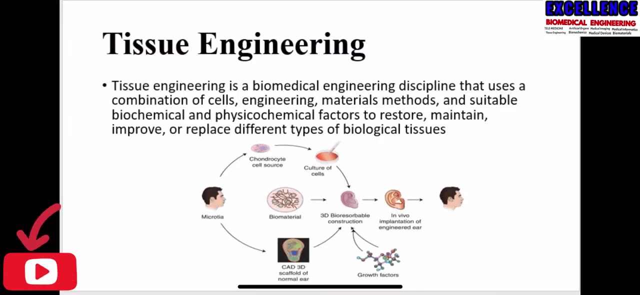 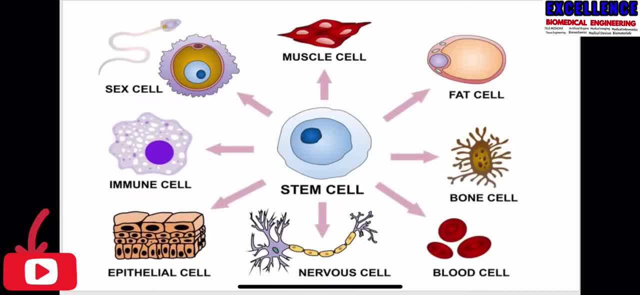 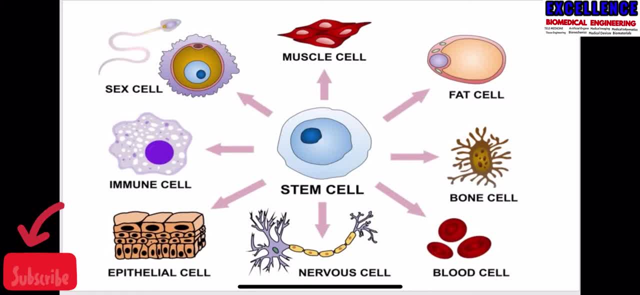 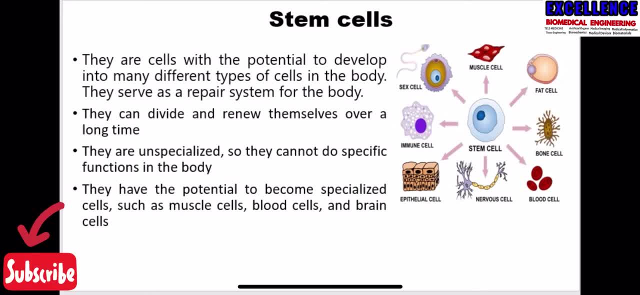 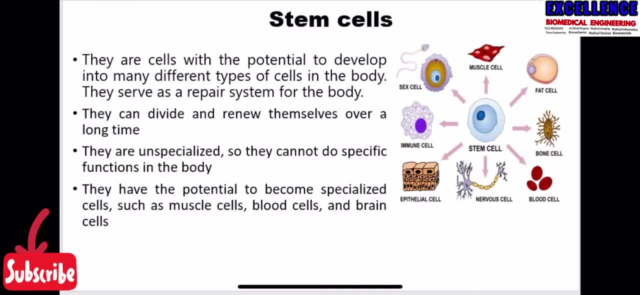 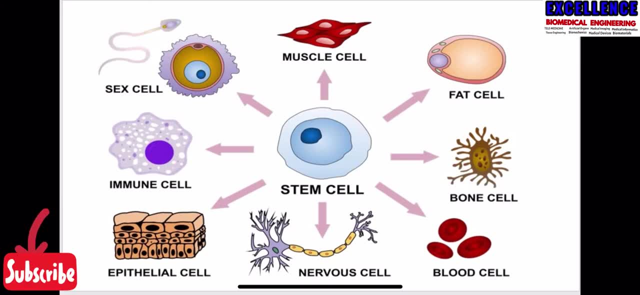 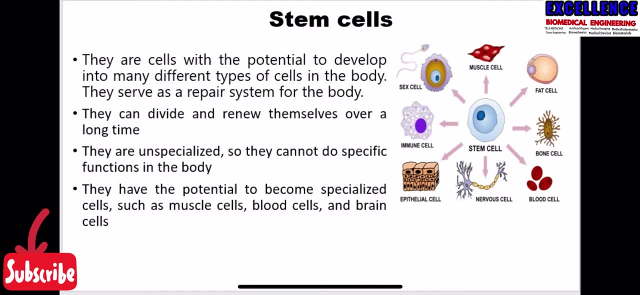 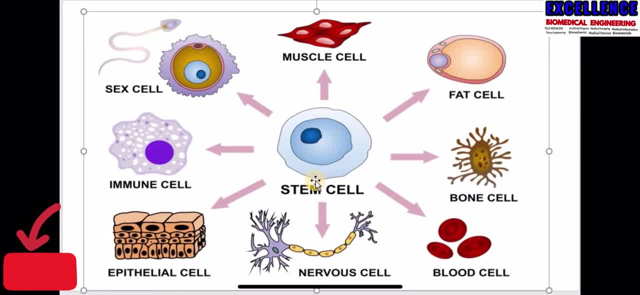 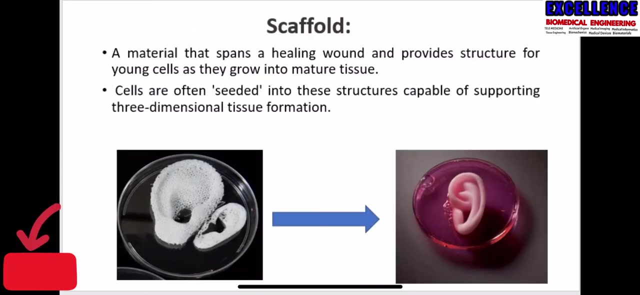 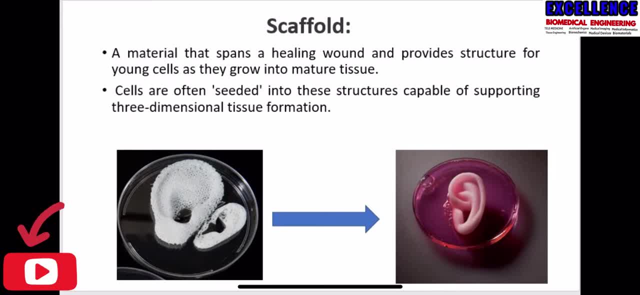 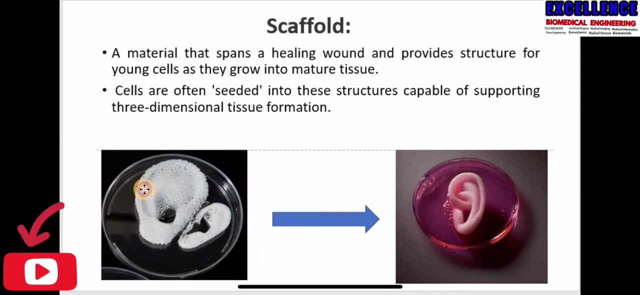 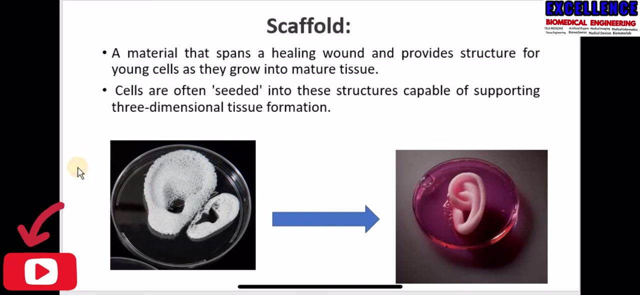 that spans a healing wound and provides structure for young cells as they grow into immature cells. you know, cells are often seeded into these structures capable of supporting three-dimensional tissue formation. as you can see from here for here, this is a polymeric, bio polymeric material, that is, you know, set into a shape of earlobe and 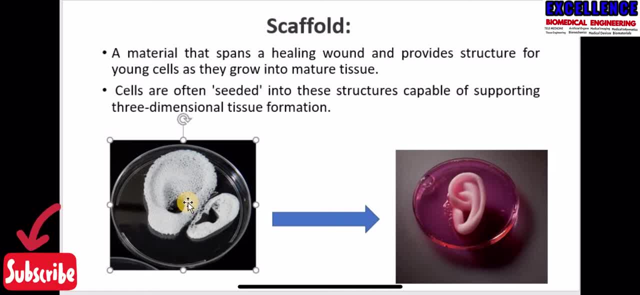 thereby we implant our stem cells into this scaffold and with time, due to the structure on which you mount them on, with time, as we are providing the growth factors, the required temperature and the required nutrients, so with time it will become like a normal earlobe, based on the structure, based on what the 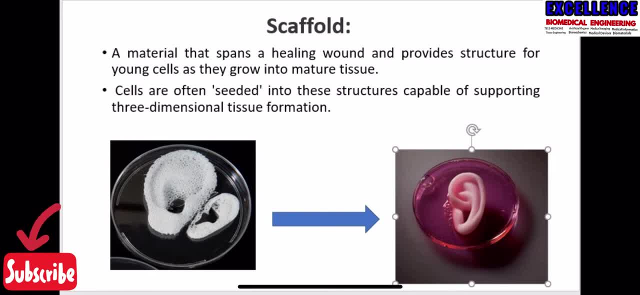 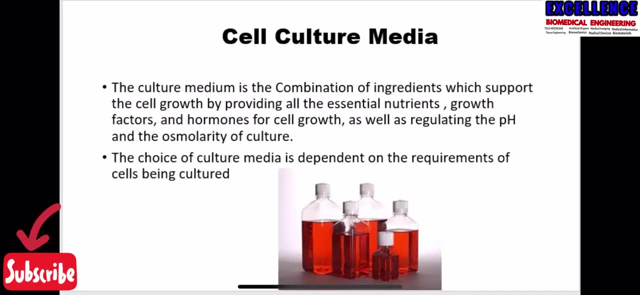 structure of the scaffold. so, and the next time we should understand from here is that we have cell culture media. the culture medium is the combination of ingredients which support the cell growth by providing all the essential nutrients, the growth factors and hormones for cell growth, as well as 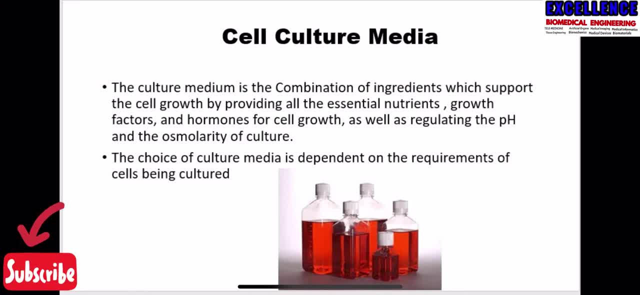 regulating the pH and the osmolarity of cell, of a sorry of of cultural. so the choice of culture media is dependent on the requirement of cells being been cultured and we have different types of cell culture media in depending on the requirements. you know it depends on the type of culture you want to make. 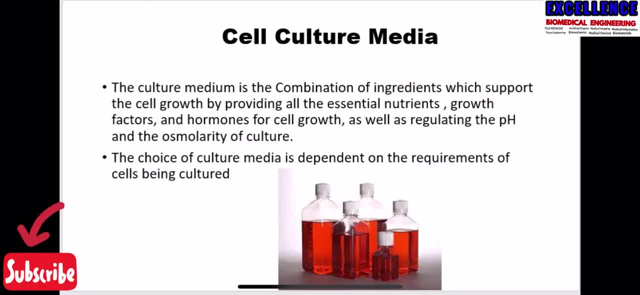 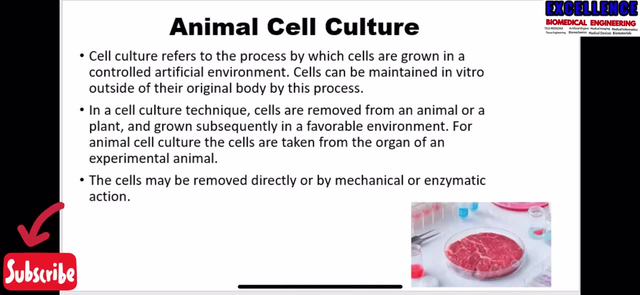 depending on the cultural media that you need. So the next one I would like to talk about here is about animal cell culture. Well, cell culture refers to the process by which cells are grown in a controlled artificial environment. Cells can be maintained in in vitro outside of their original body by this process. 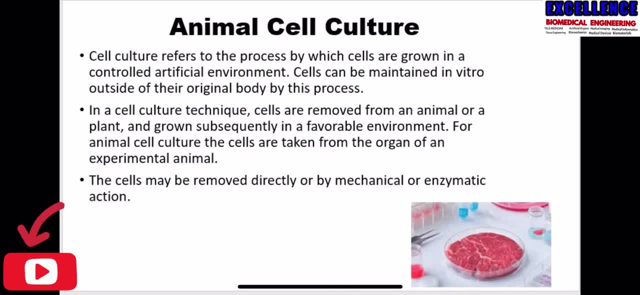 So in cell culture techniques, cells are removed from an animal or a plant and grown subsequently in a favorable environment for animal cell culture. The cells are taken from the organ of an experimental animal, Just like the previous slide that we showed earlier, where we show someone like here: 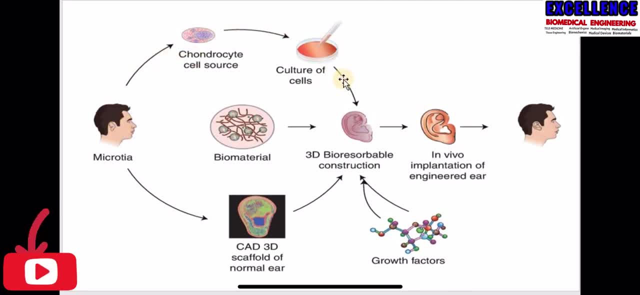 this is human. so the stem cells are removed from here, and then there will be growth factors and other nutrients, all together cultured, put on inside a scaffold, and with time it will grow on that scaffold and become a complete organ. So the next thing I would like to talk about is cell line. 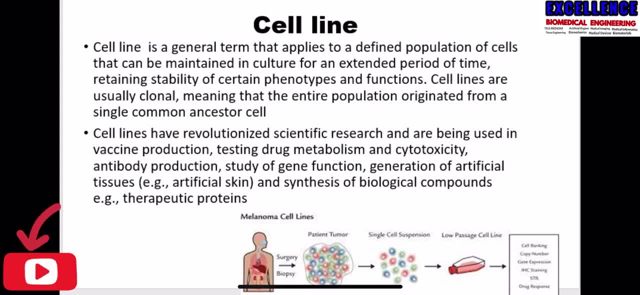 Well, cell line is a general term that applies to a defined population of cells that can be maintained in culture. So cell line is a general term that applies to a defined population of cells that can be maintained in culture for an extended period of time, retaining stability of certain phenotypes and functions. 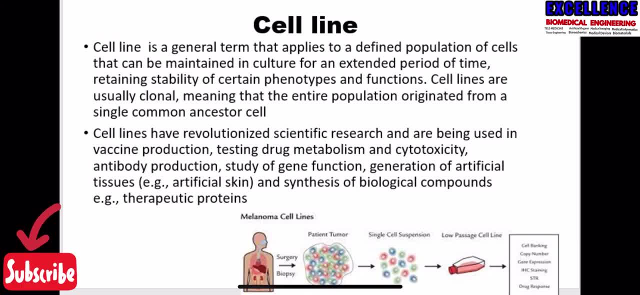 Cell lines are usually clonal, meaning that the entire population originated from a single common ancestor cell. So cell lines have revolutionized specific research and are what have been used in vaccine production, testing, drug metabolism and cytotoxicity check, antibody production, study of gene function. 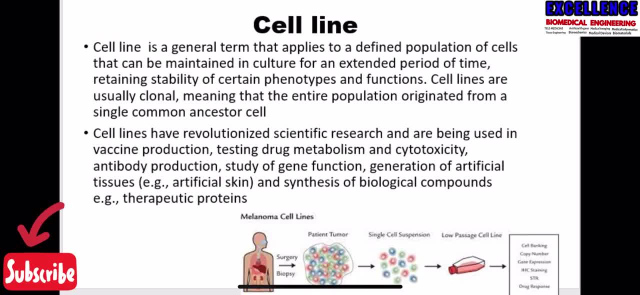 generation of artificial tissues, like, example, artificial skin- we have the ear lobe also- and then synthesis of biological compounds- example, therapeutic proteins, Because we have a situation where we need some specific proteins that maybe someone is lacking. For example, let me take the example of insulin. 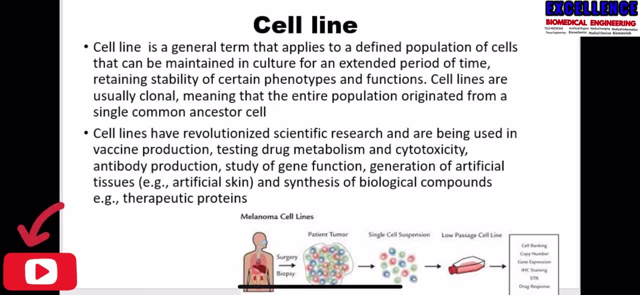 Now, people who are diabetic. Now, people who are diabetic, they have this inadequacy of producing proper insulin. So what we do? we get cells that are capable of producing insulin. We culture them in the lab. So we made a cell line of these cells. 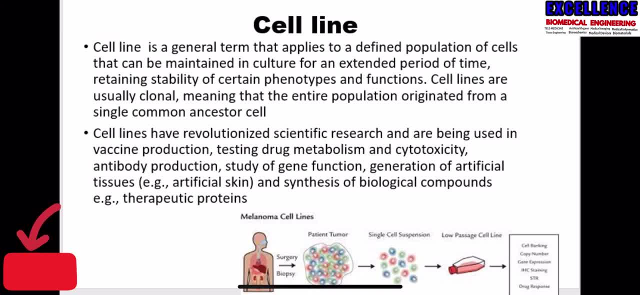 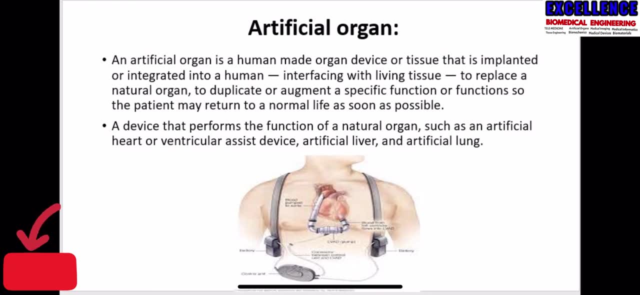 Thereby they will be producing insulin for us in the lab and we will be selling it out in the market. So the next thing I would like to talk about is artificial organ. As you all know, we are talking about tissue engineering, so it is very important we should talk about artificial organ. 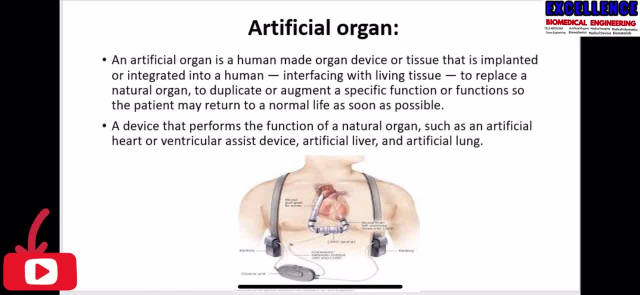 Artificial organ is a human-made organ, device or tissue that is implanted or integrated into a human interfacing with living tissue to replace a natural organ or to duplicate or augment a specific function or functions so the patient may retain to a normal life as soon as possible. 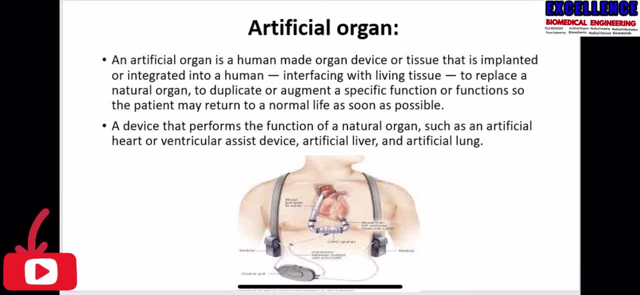 So a device that performs the function of a natural organ, such as an artificial heart or ventricular acid device, artificial liver and artificial lung are all termed as artificial organs. So in tissue engineering there is one thing also we need to understand, which is aseptic technique. 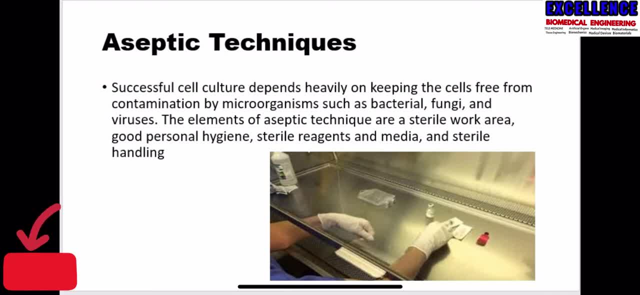 Well, no matter the ability of cell to divide and everything, if there is no aseptic technique in the process, it is not going to work. So successful cell culture depends heavily on keeping the cell free from contamination by microorganisms such as bacteria, fungi and viruses. 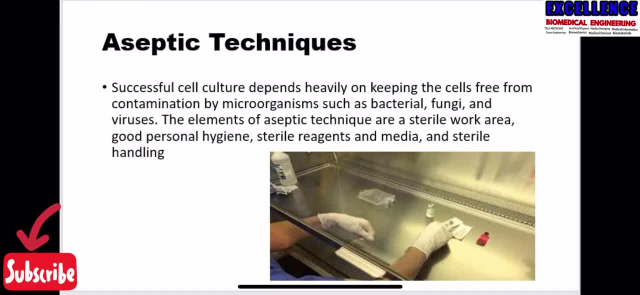 The elements of aseptic techniques are a sterile work area, good personal hygiene, sterile reagents and media and sterile handling. So that's why we are talking about aseptic techniques. That is why in tissue engineering lab you have some equipment like laminar hood. 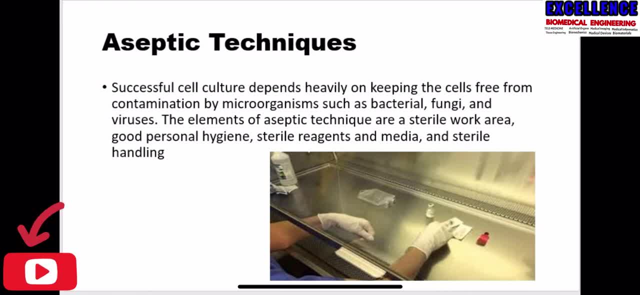 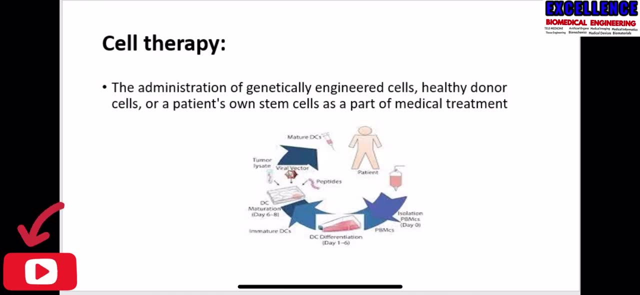 and some other equipment that will prevent bacteria or fungi from entering our cells while we are carrying out the tissue culture process. So the next terminology I will talk about is cell therapy. Cell therapy is just simply the administration of genetically engineered cells- Healthy donor cells or patients own stem cells- as a part of medical treatment. 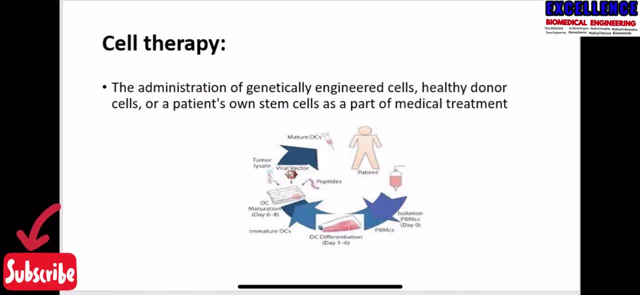 For example, someone who has a problem with his skin is chopped off by a knife or through accident, So now you need to patch that place due to the hole that is made is too deep. So cell therapy is the process of getting his cells grow them in the lab or from the tissues there and then filling the gap. 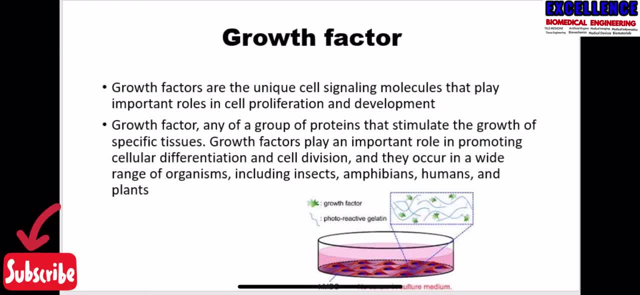 So the next I would like to talk about is growth factor. Well, growth factors are the unique cell signaling molecules that play important roles in cell proliferation and development. Growth factors are any of a group of proteins that stimulate the growth of specific tissues. 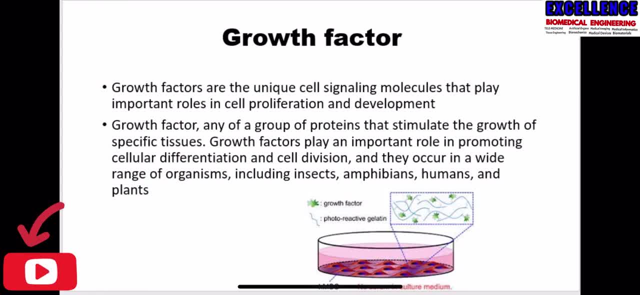 Growth factors play an important role in promoting cellular differentiation and cell division, and they occur in a wide range of organisms, including insects, amphibians, humans and plants as well. So with this we have come to the end of this lecture. It is very important that we cut it short. 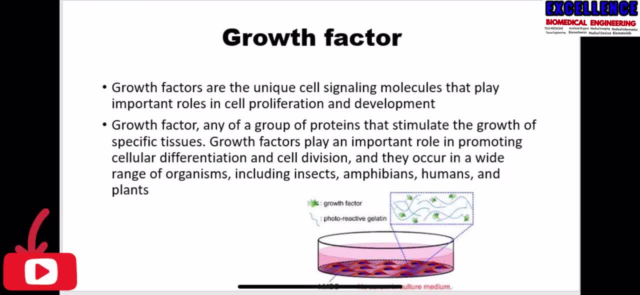 We will be making series of this lecture, So this is the part one Please don't forget to like. if this is your first time on this YouTube channel, Support our video by liking our video, subscribing to our channel and sharing the video as well. Thank you.